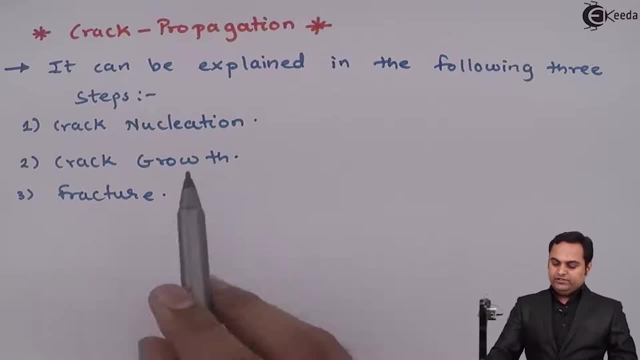 hole to a very high value. So in that there are three stages: Crack Nucleation, Crack Growth and Fracture. So for that here I will explain. the detailed explanation is as follows. So the first one is Crack Nucleation. Now for Crack Nucleation. 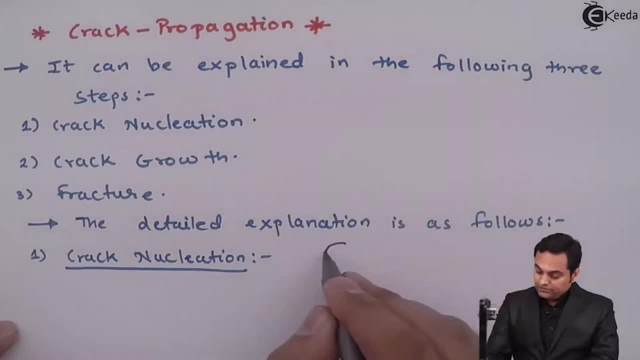 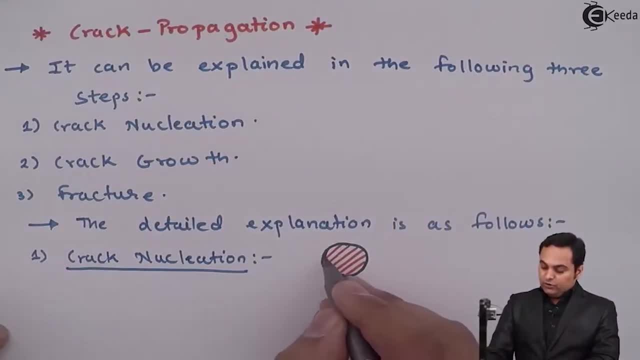 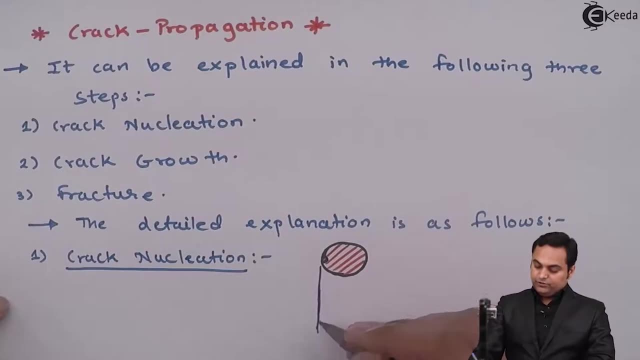 is meant by Crack Nucleation. In this there is a small hole inside the element, and if I project this here, I am drawing the two views. So now, suppose this is the front view of the component, and here we have, suppose this is the top view. 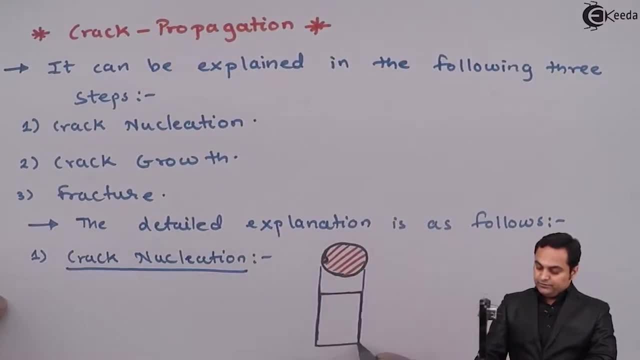 And here is the front view of the component. Then, in case of Crack Nucleation, at first there is a small cavity, a very small hole or a crack which is there inside a material. So Crack Nucleation it means that the failure will begin at a small nucleus. So this is 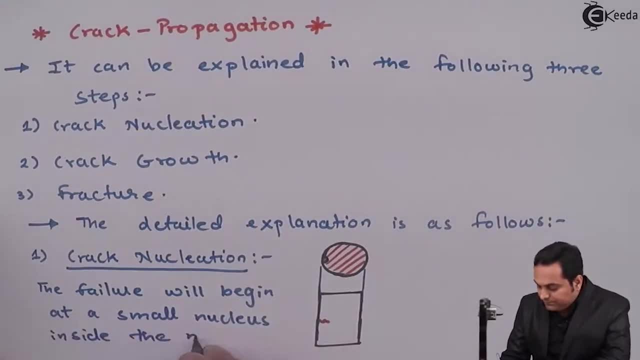 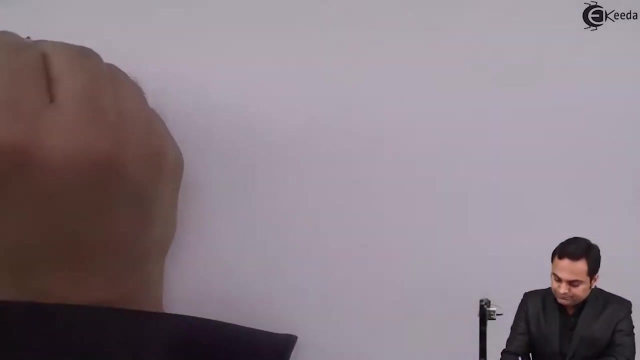 Crack Nucleation. So this is Crack Nucleation inside the material, inside it. if we have a small hole or cavity and when the load is applied externally to the material, then crack will start forming from this small hole which is present inside. Next, Crack Growth For. 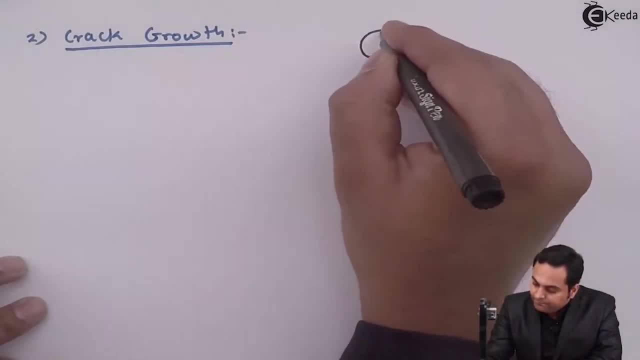 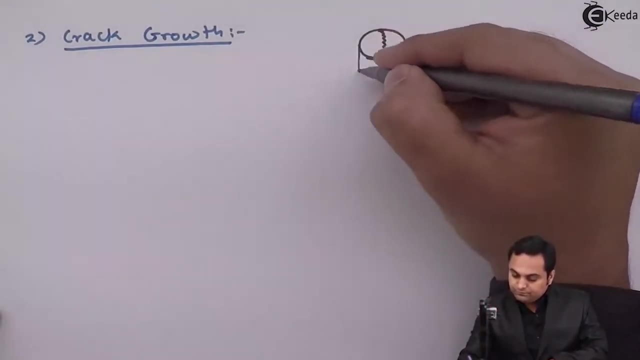 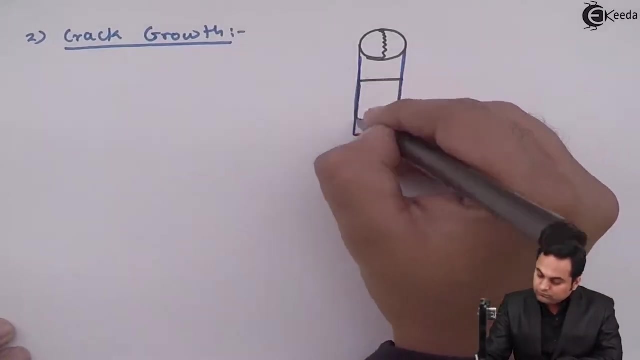 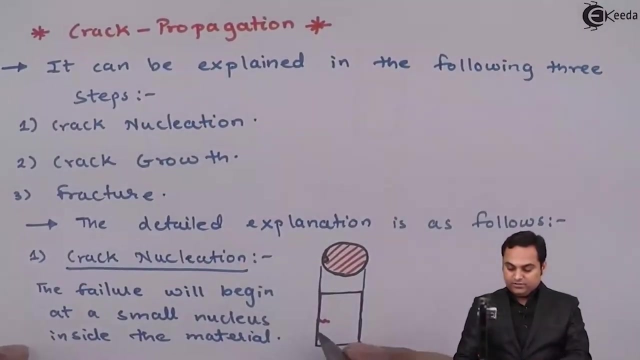 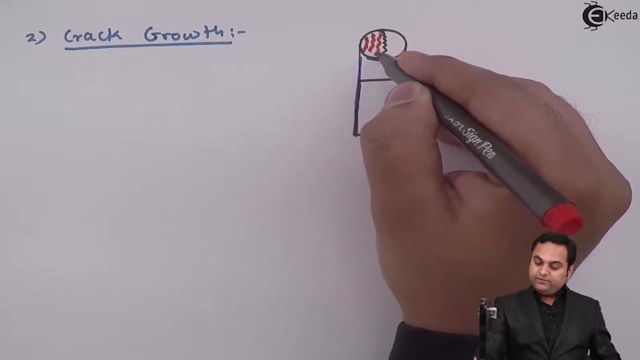 that also. I will draw the diagram and explain. Now, in case of crack growth, once the nucleus is formed, that is, a hole is present, then the crack will go on increasing. that is, the cracks which are developed inside. the material will go on increasing, and this is the direction. 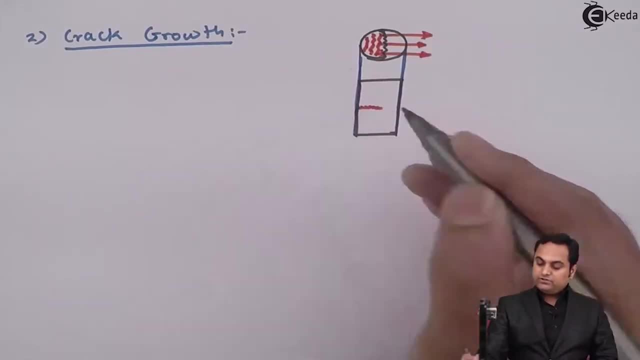 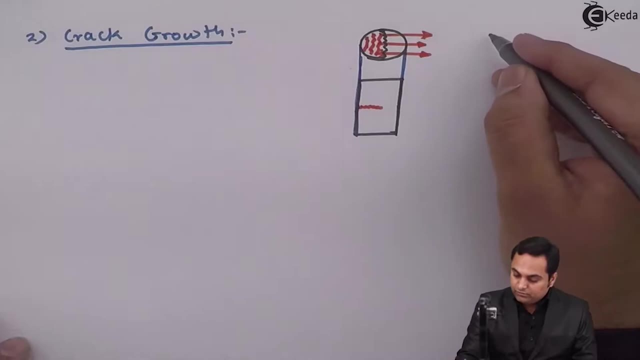 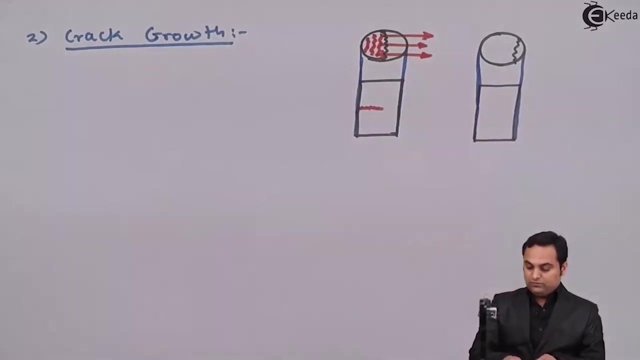 of the crack, So it becomes large. Next, after that again, if we go on increasing the load now, when the load is increased again, then the crack which is moving in the direction towards right, the cracks, would go on increasing internally and it will reach up till there. 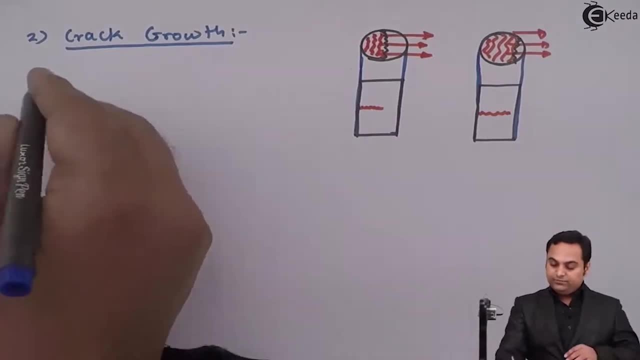 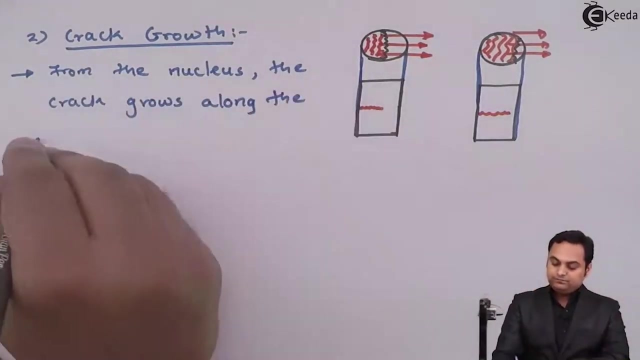 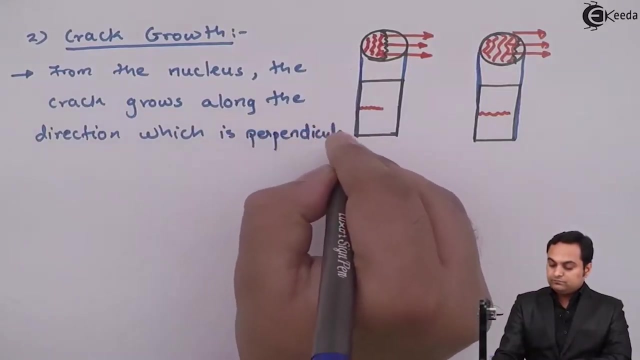 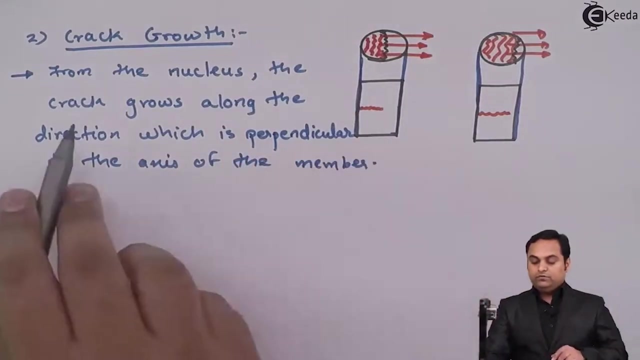 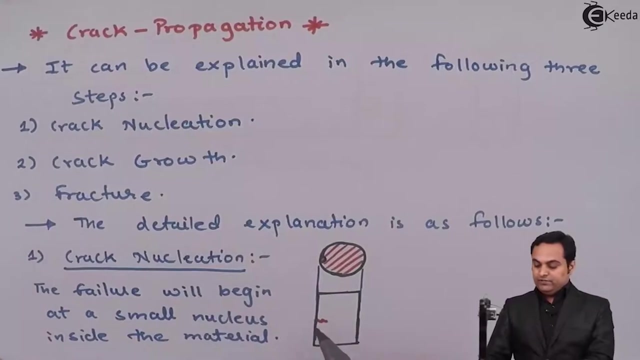 In case of crack growth. here I can write down that from the nucleus the crack grows along the direction which is perpendicular to the axis of the member. So from the nucleus, as we have seen in case of the crack propagation, the first step was crack nucleation from this small hole. when the load is applied externally, failure will 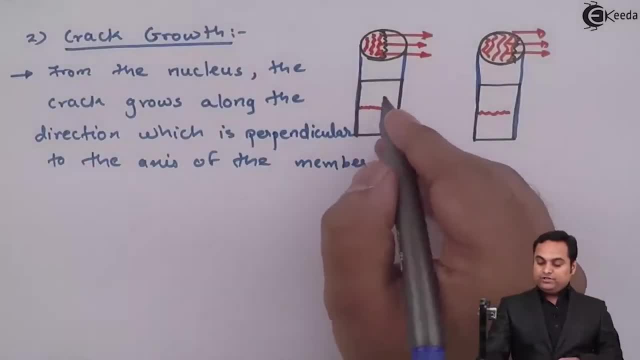 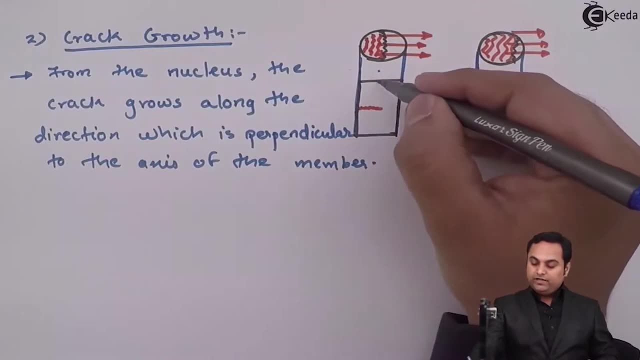 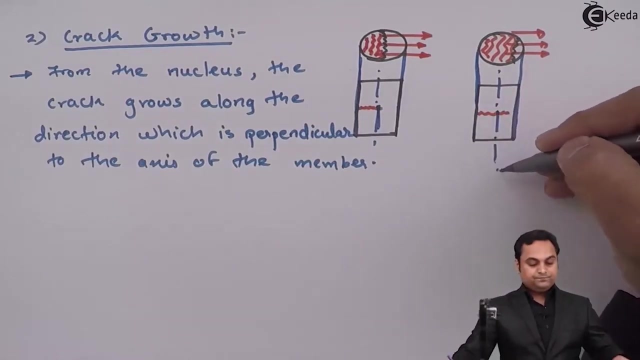 start from this nucleus And it will Go on progressing, that is, the crack will go on increasing in a direction. that is the direction which is perpendicular to the axis- here is the axis of the member. So, perpendicular to this axis, the crack is formed.